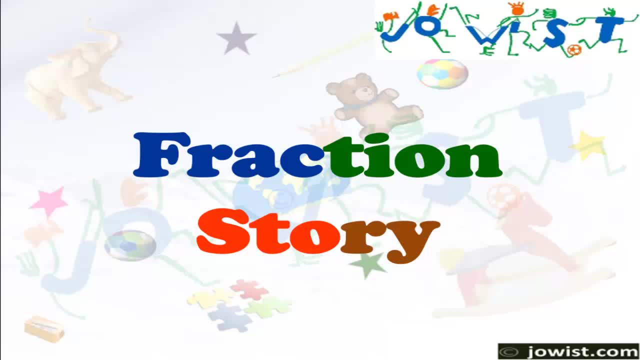 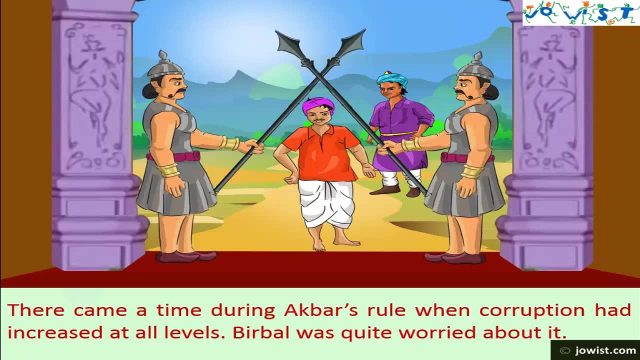 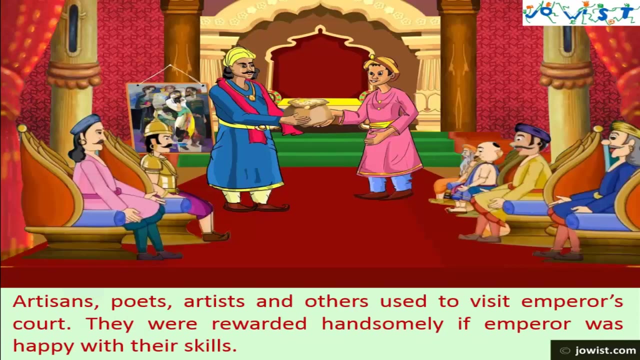 FRACTION STORY. There came a time during Akbar's rule when corruption had increased at all levels. Birbal was quite worried about it. Artisans, poets, artists and other used to visit emperor's court. They were rewarded handsomely if emperor 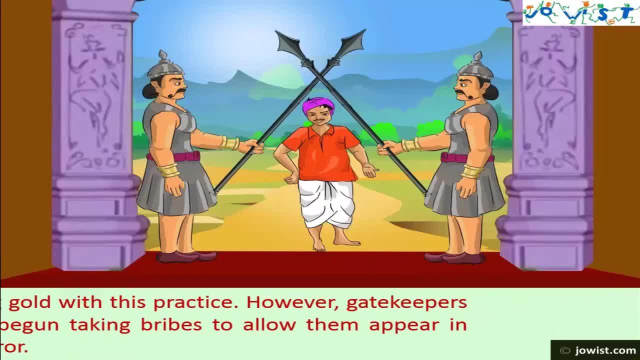 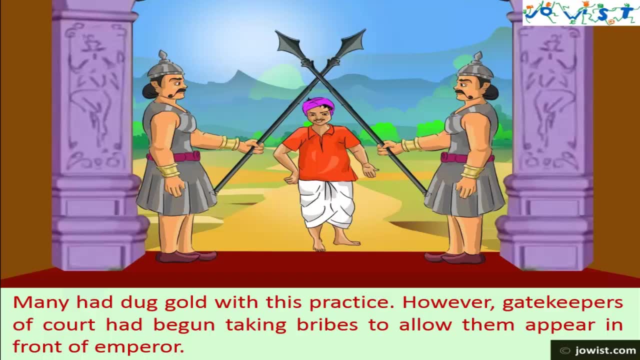 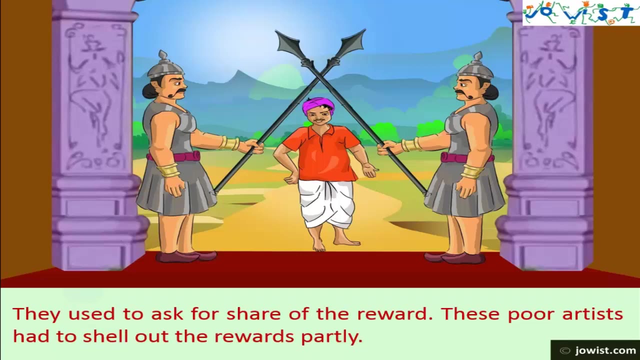 was happy with their skills. Many had dug gold with this practice. However, gatekeepers of court had begun taking bribes to allow them appear in front of the emperor. They used to ask for the share of the reward. These poor artists had to shell out the rewards. 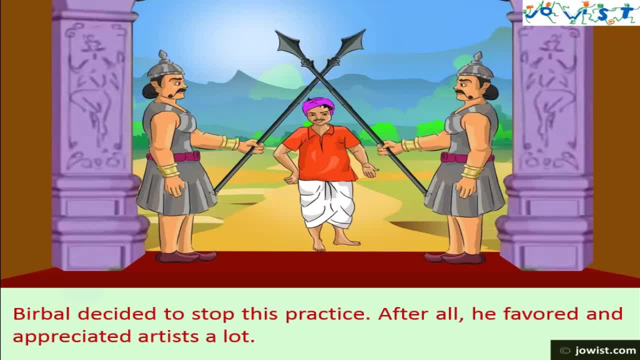 partially. Birbal decided to stop this practice. FRACTION STORY: There came a time during Akbar's rule when corruption had increased at all levels. Birbal had quite a lot of artisans After all. he favored and appreciated artists a lot. One day, guards found an old brahmin seeking permission. 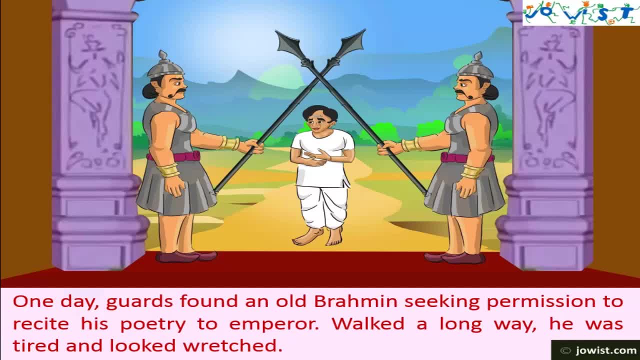 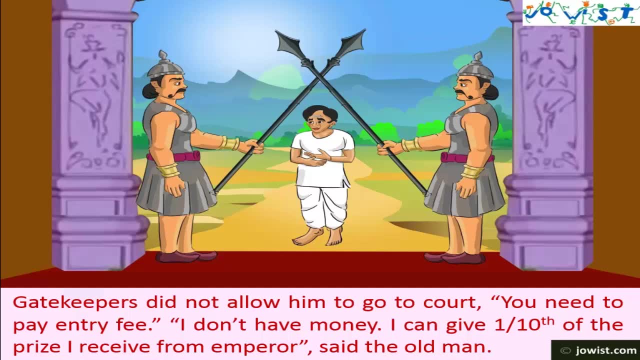 to recite his poetry to emperor Walked the long way. he was tired and looked wretched. Gatekeepers did not allow him to go to the court. You need to pay entry fee. I don't have money. I want to go to the court, But I can't without money and I don't have money. 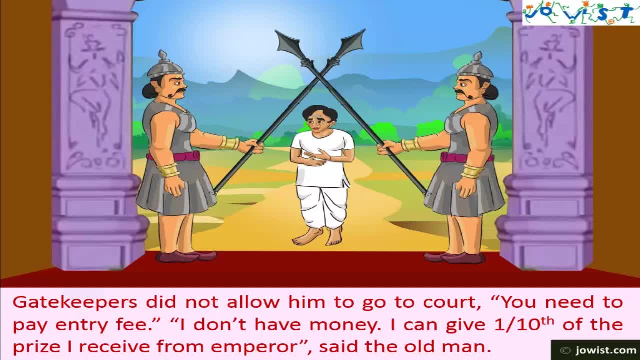 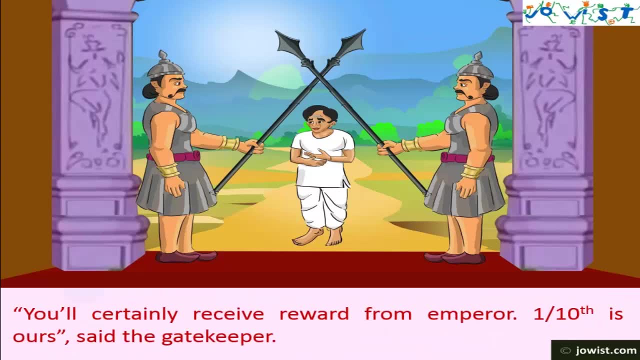 I can give one-tenth of the prize I received from emperor, said the old man. You will certainly receive reward from emperor. One-tenth is ours, said the gatekeeper. When the old man went inside, the gatekeeper said his fellow. 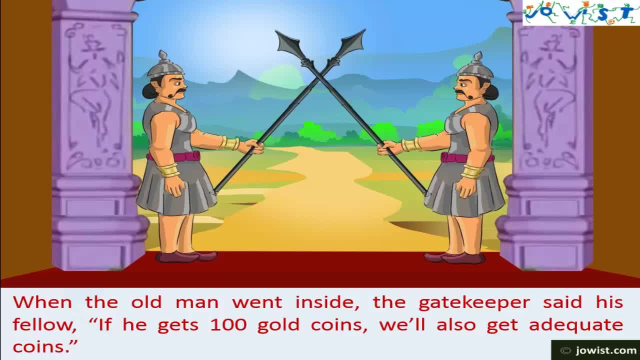 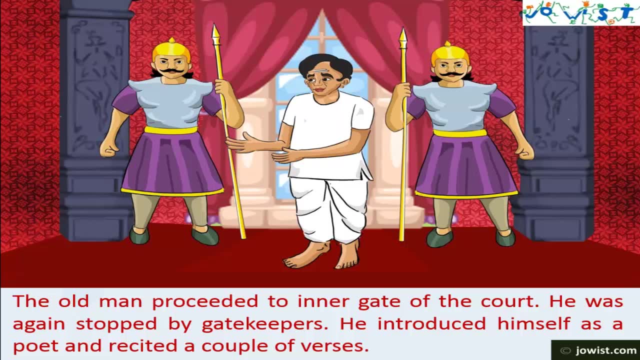 If he gets hundred gold coins, we will also get adequate coins. The old man proceeded to inner gate of the court. He was again stopped by the gatekeepers. He introduced himself as a poet and recited a couple of verses. Guards appreciated his poem. Your verses seem to be good. We hope you get a fair reward.